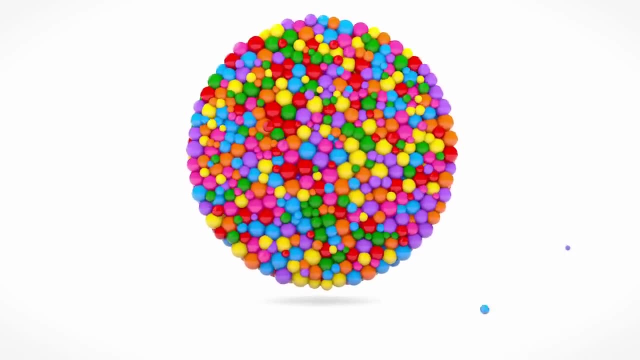 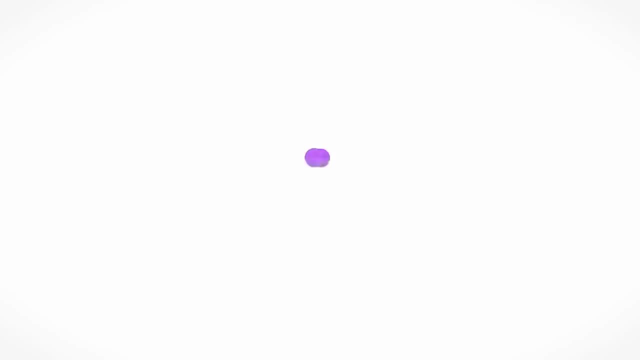 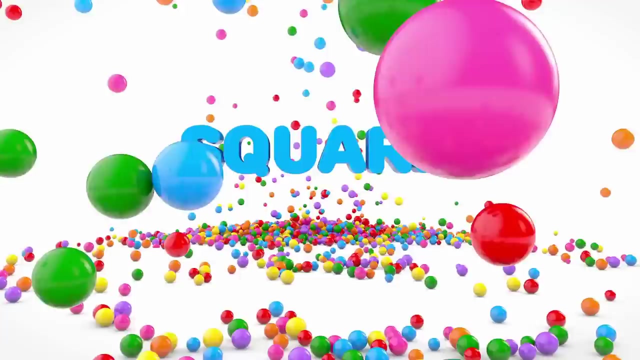 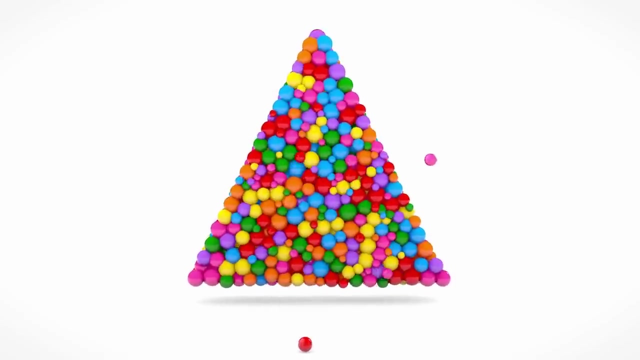 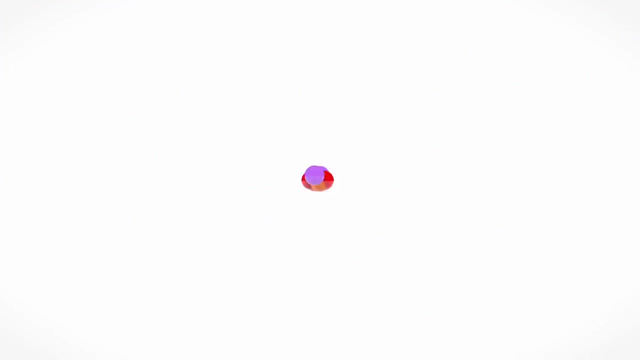 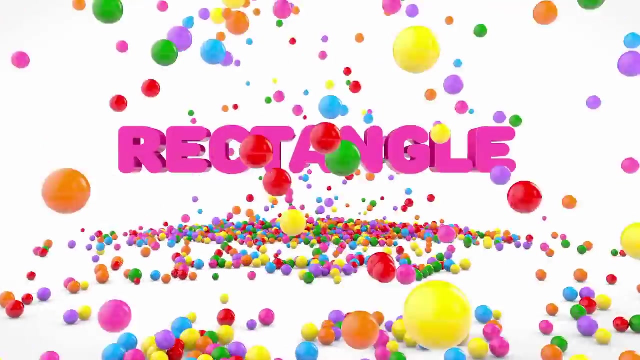 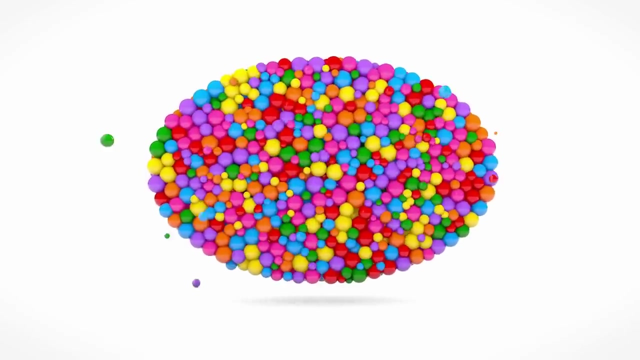 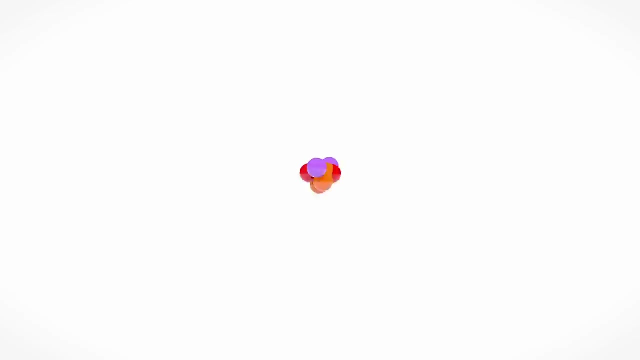 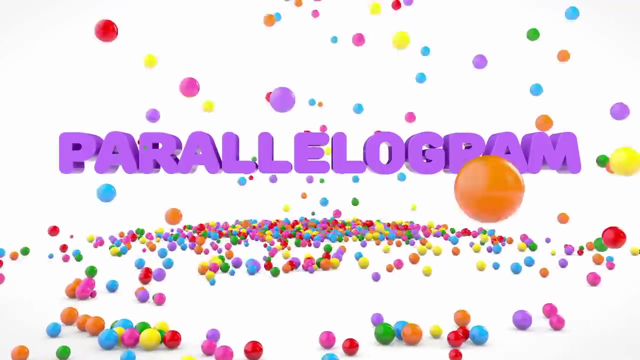 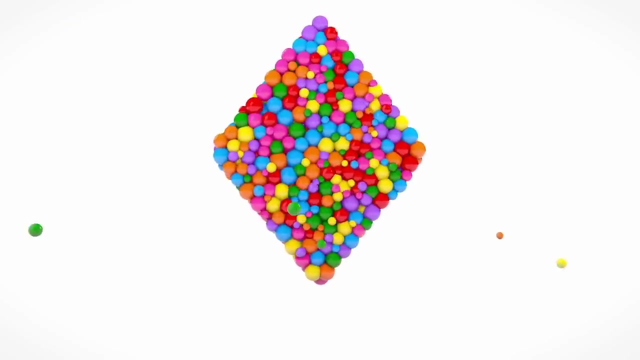 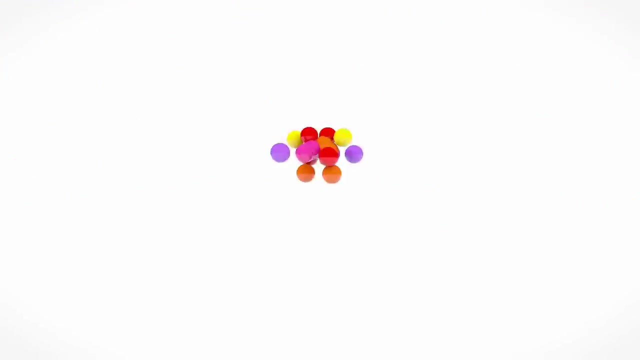 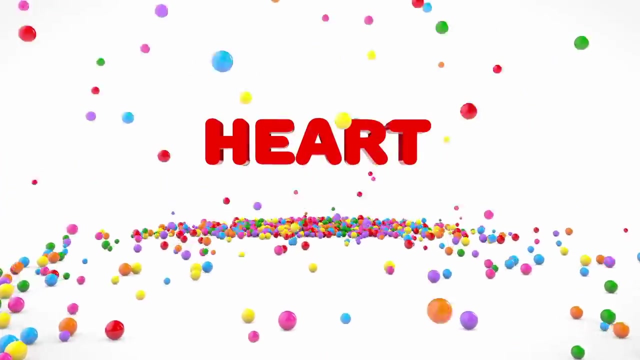 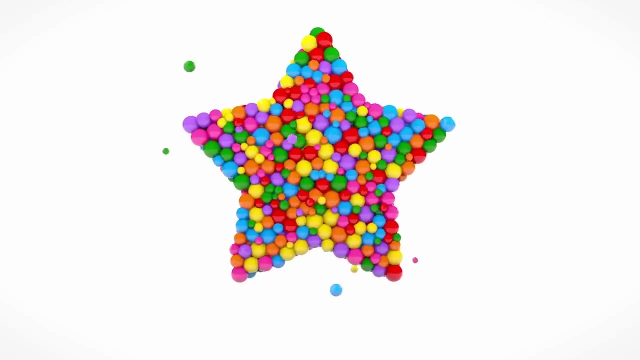 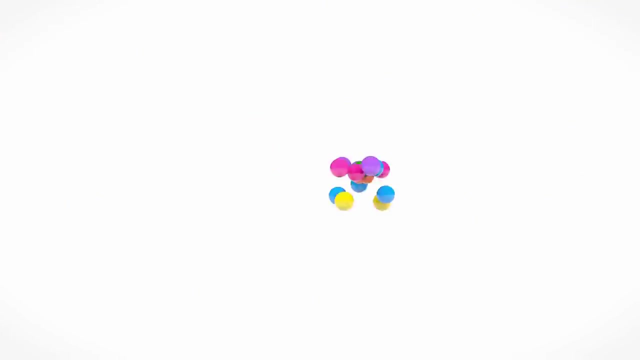 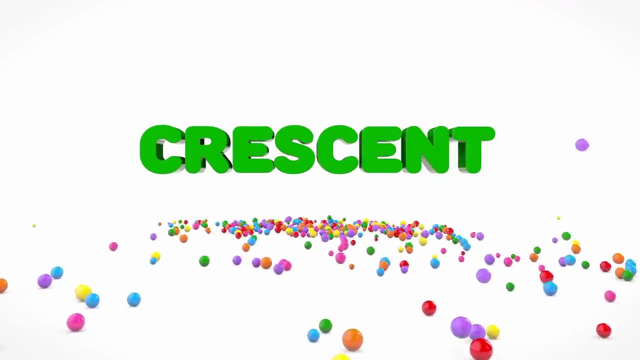 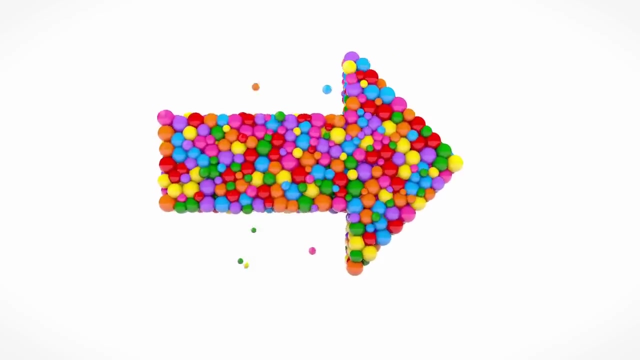 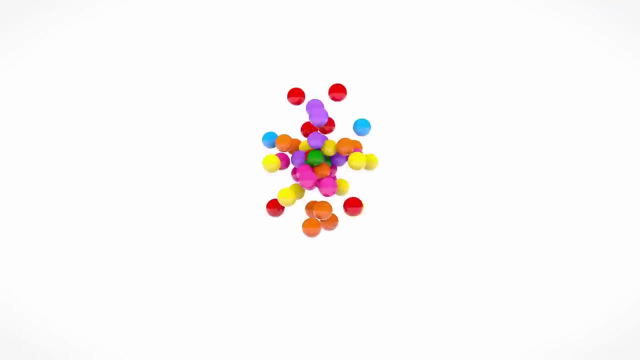 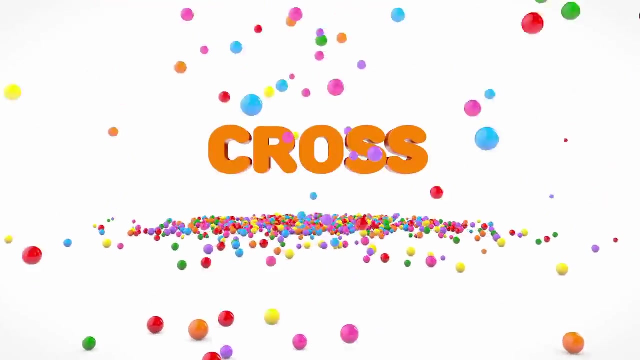 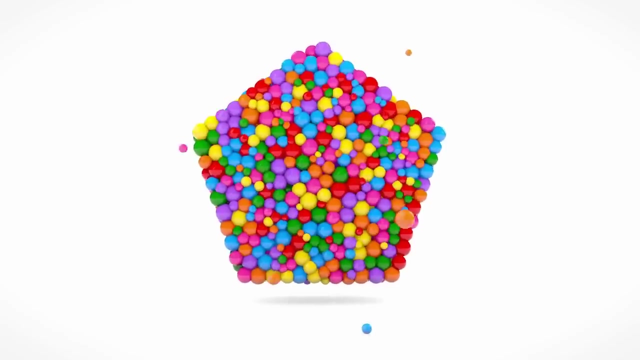 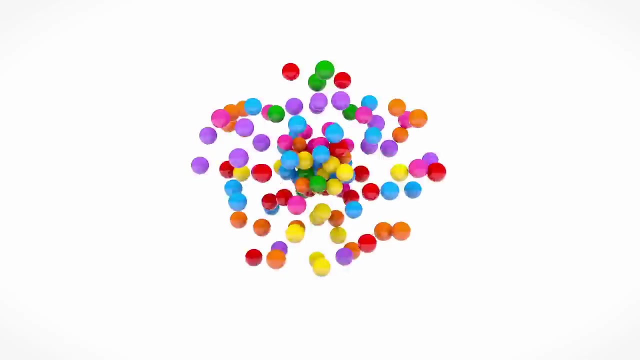 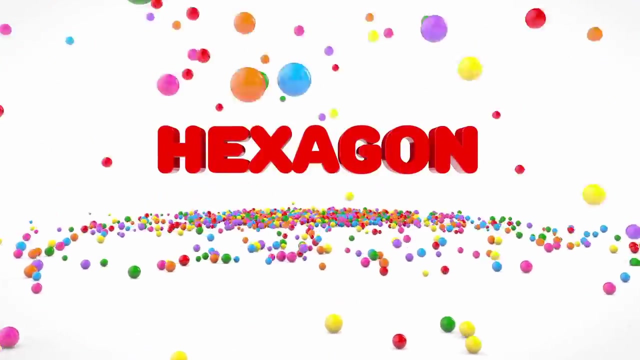 circle, square, triangle, triangle, rectangle, oval, oval, parallelogram, rhombus, heart, love, small, large, large, small, large, small, small, small, inside, inside, inside, between between between, Wow, Cross, Yay, Cross. Wow, Pentagon, Yay, Pentagon, Wow, Hexagon, Yay, Hexagon. 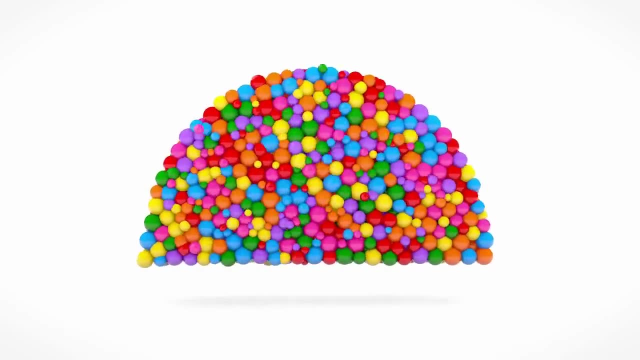 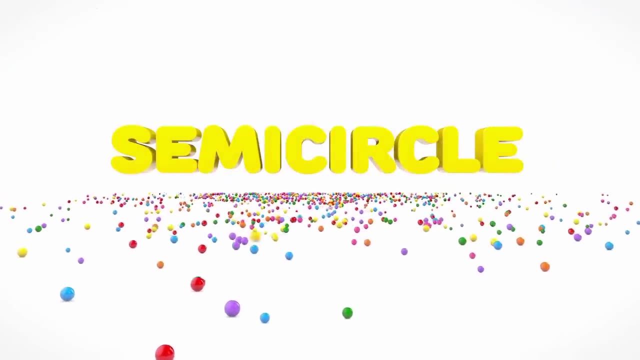 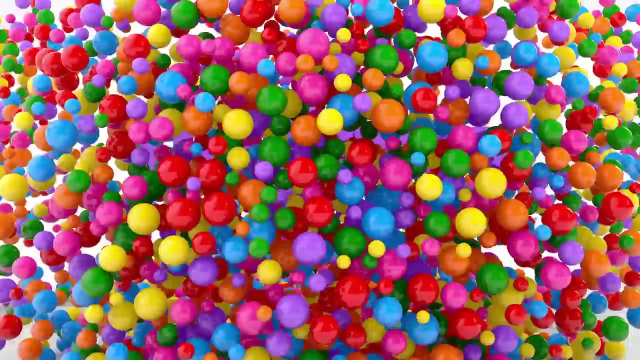 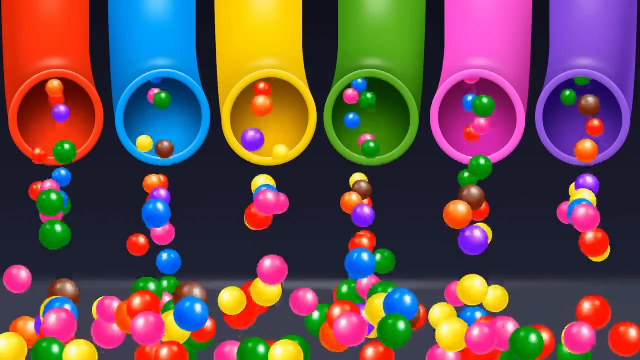 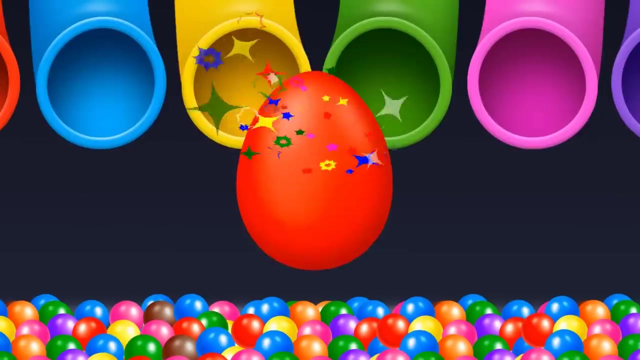 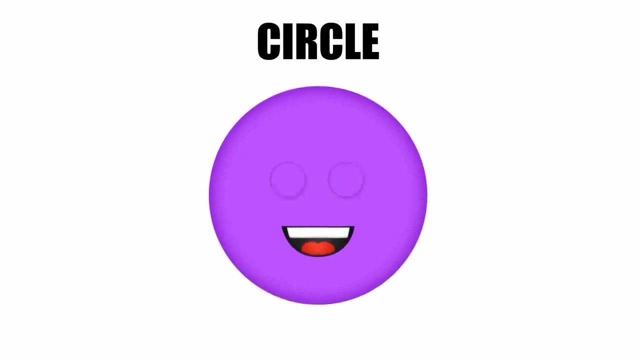 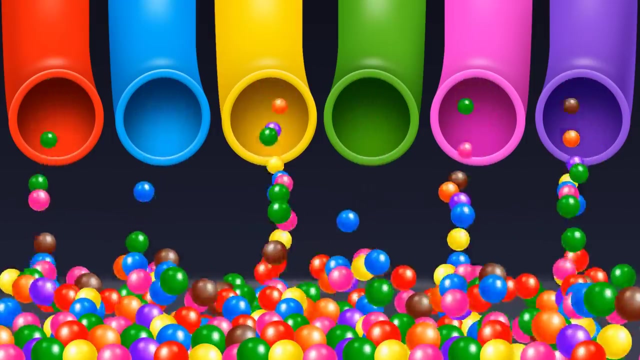 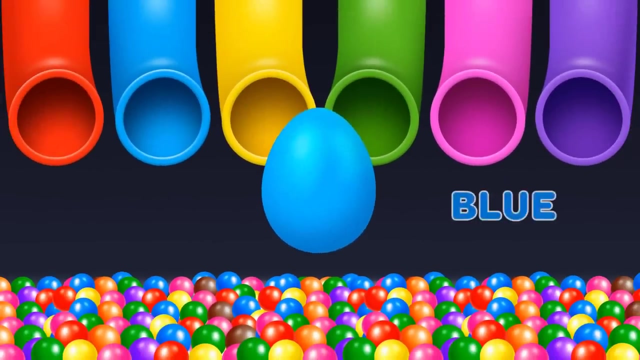 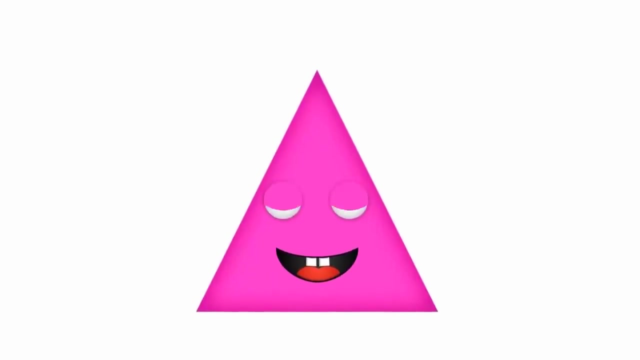 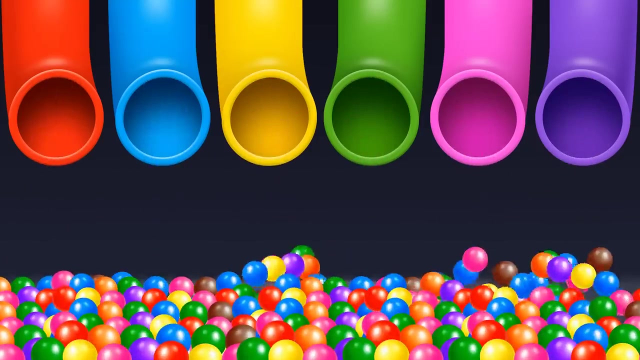 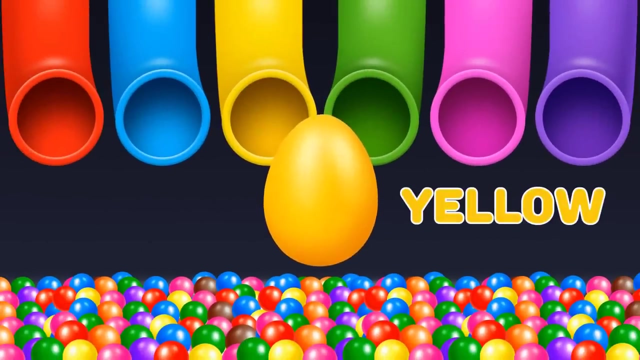 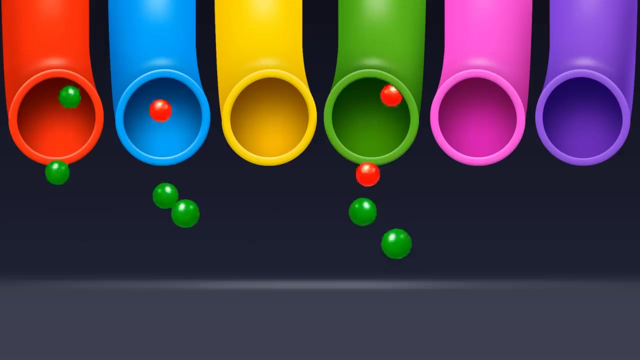 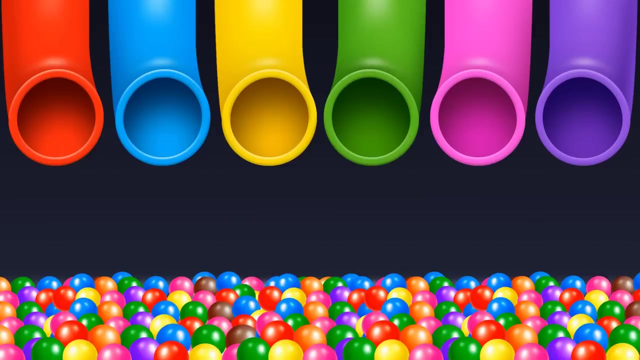 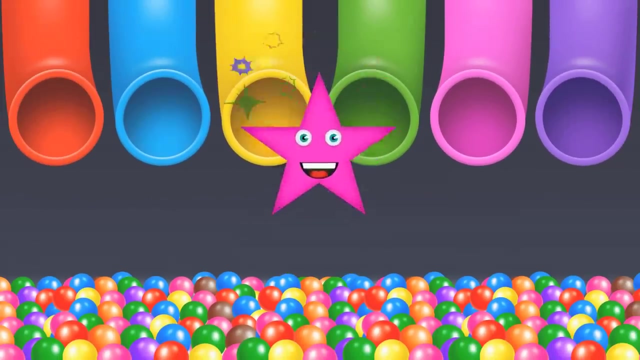 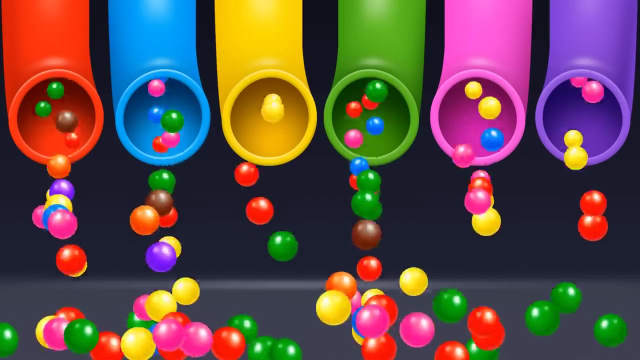 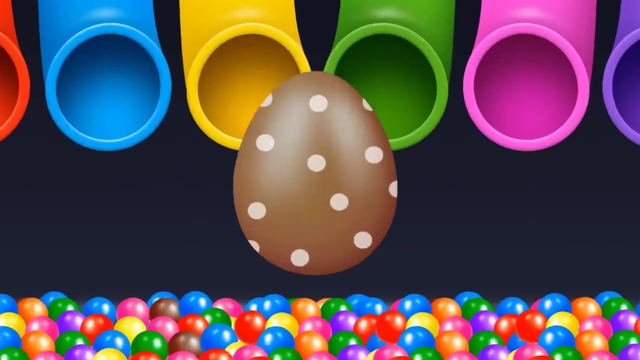 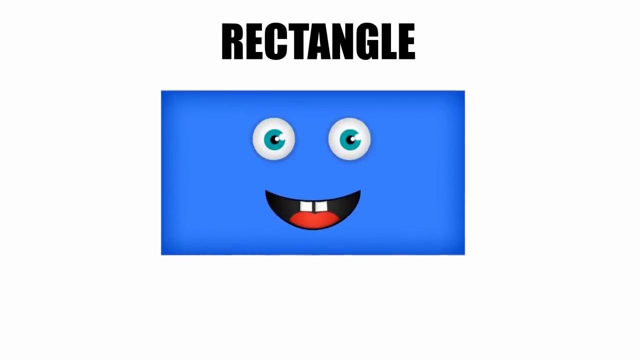 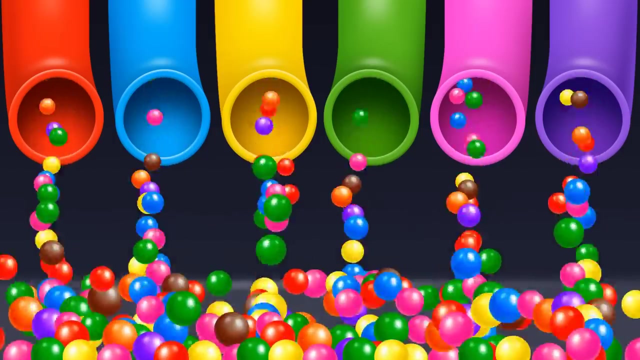 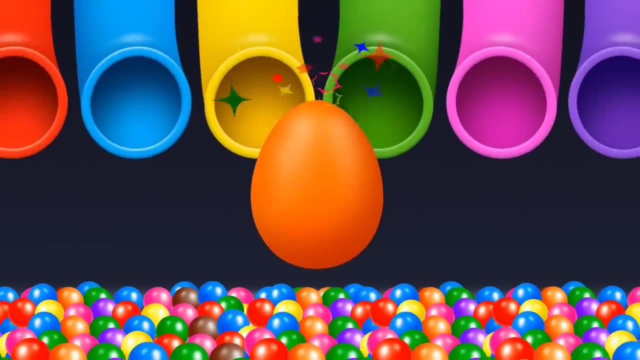 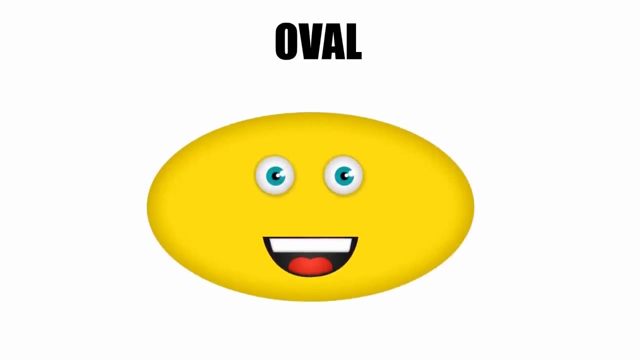 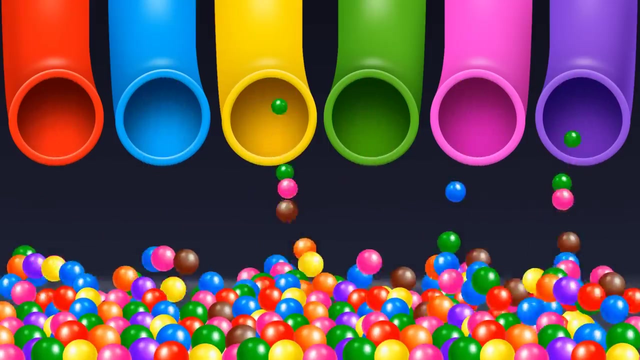 Wow, Semicircle, Yay, Semicircle. Wow, Trapezoid, Yay, Trapezoid. Red Circle, Blue Triangle, Yellow Square, Red Green Star, Pink Rectangle, Rectangle, Super definetive. Rubik's Colour: Oval, cold Blue, Brainstorming Triangle, Red ари. 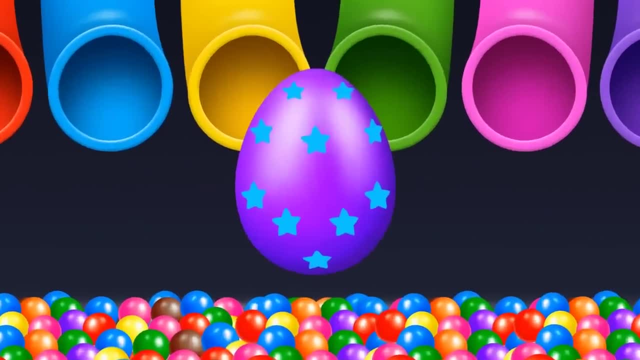 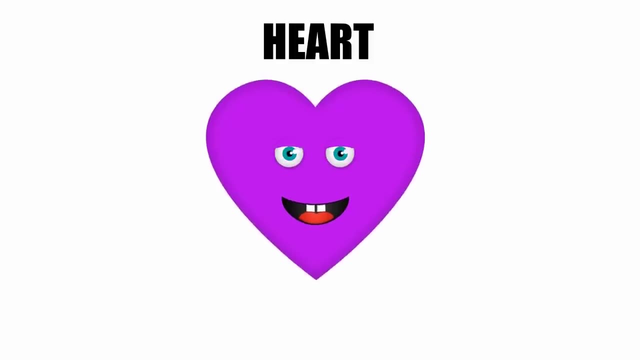 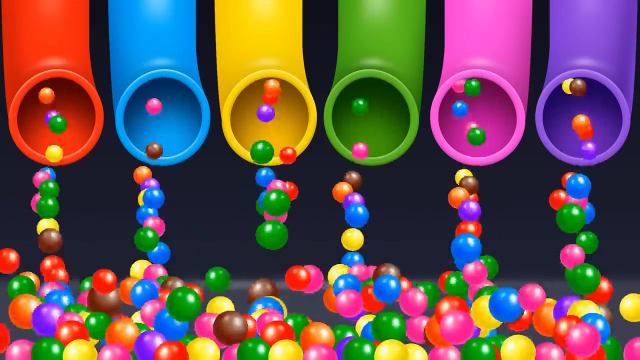 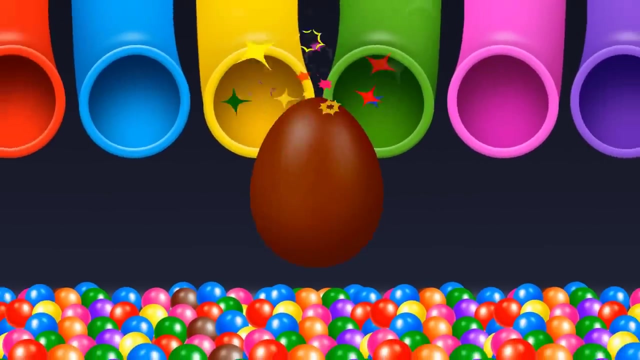 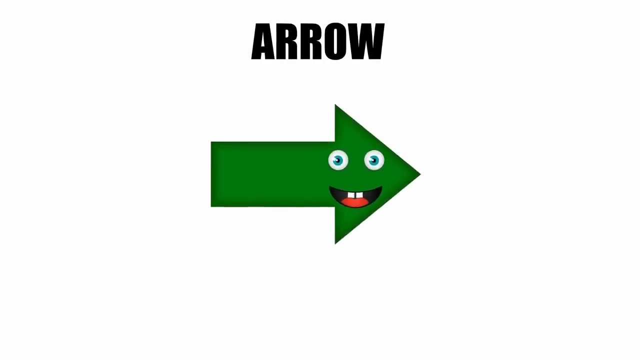 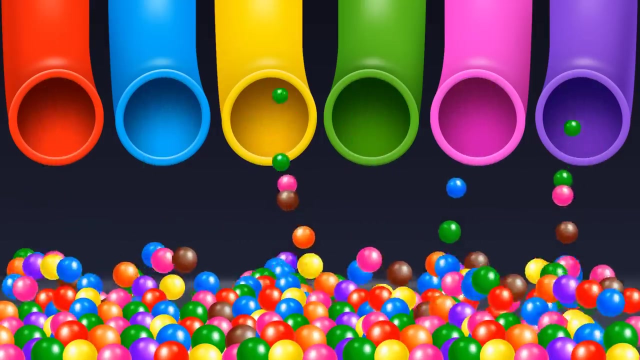 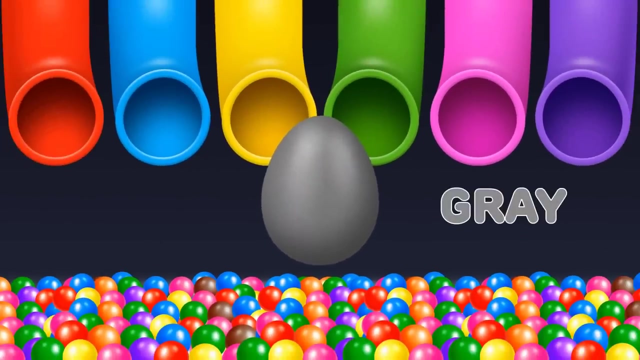 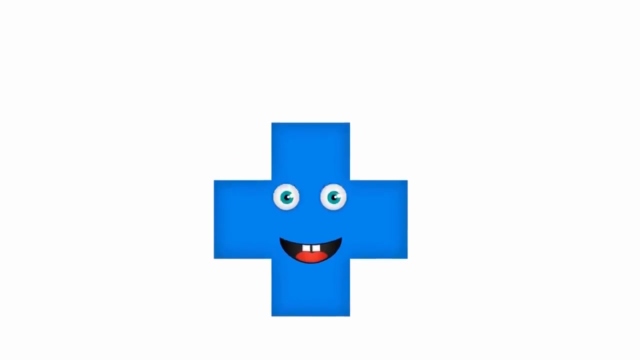 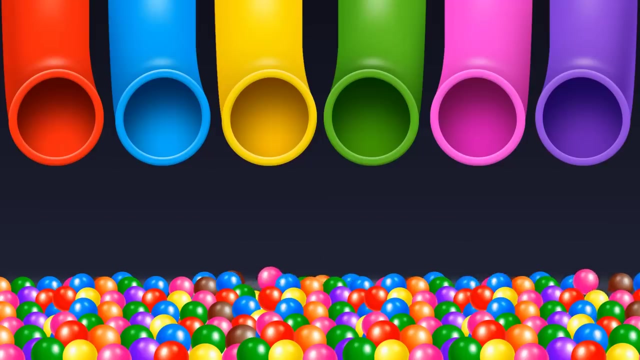 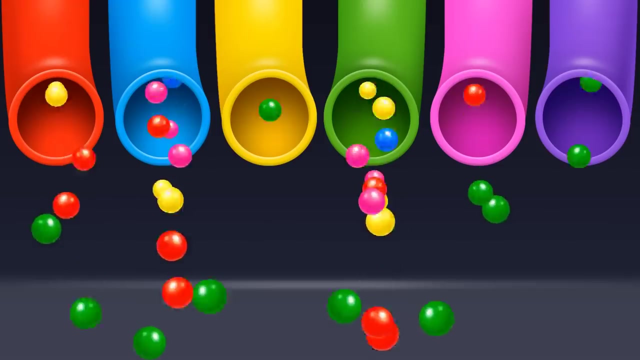 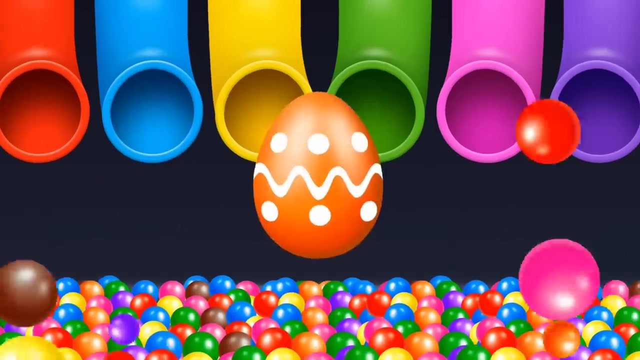 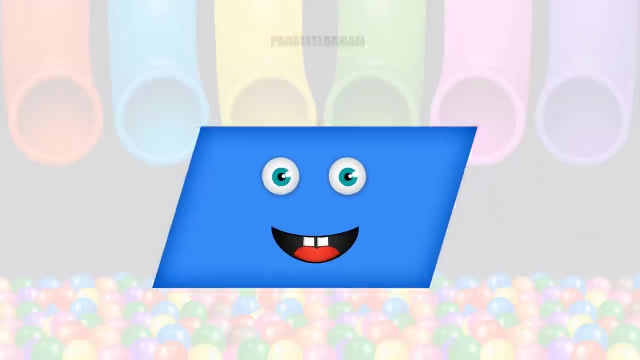 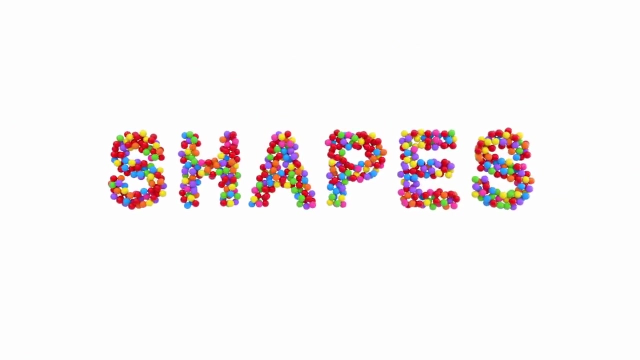 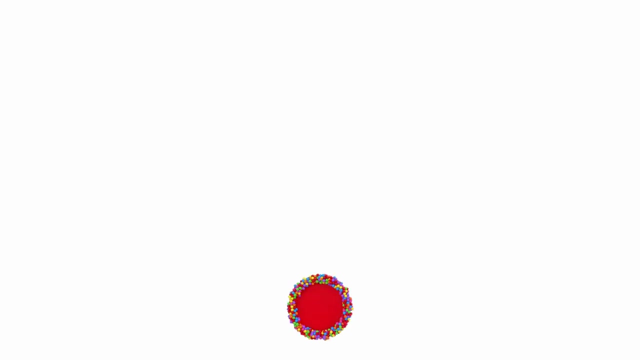 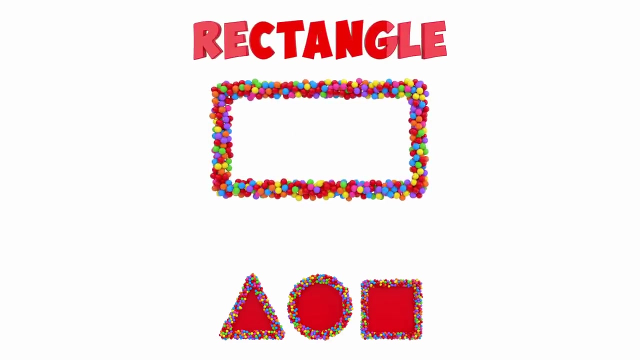 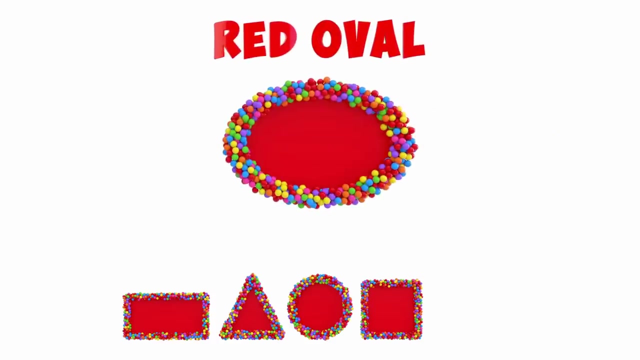 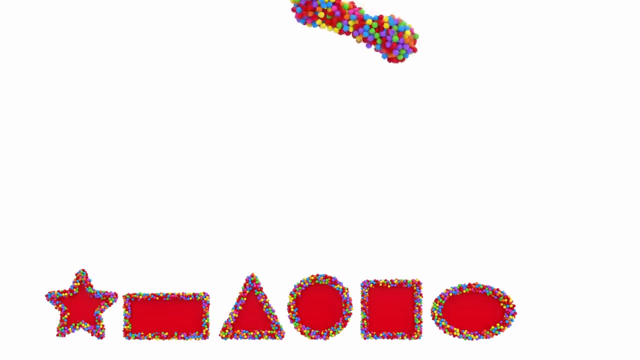 红, Red Blue- My originator. Red Purple Heart. Brown Arrow. Blue Gray Cross. White Black Crescent, Bright White. Parallelogram, Circle- Red circle. Triangle, Red triangle, Square, Red square. Rectangle, Red rectangle. Oval- Red oval Star- Red star, Rhombus, Red, rhombus Heart. 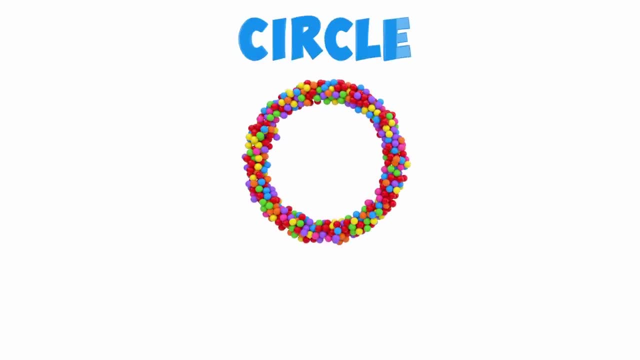 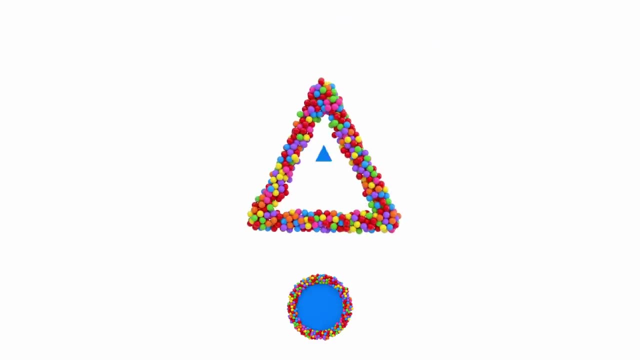 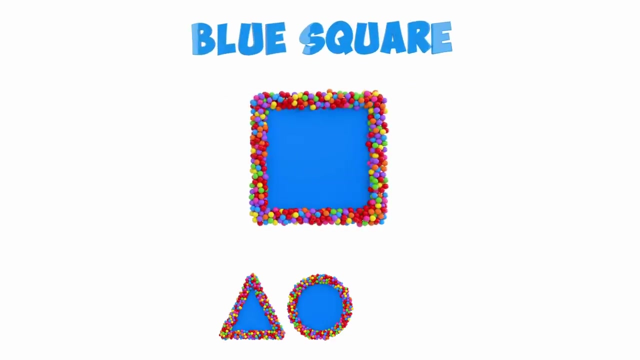 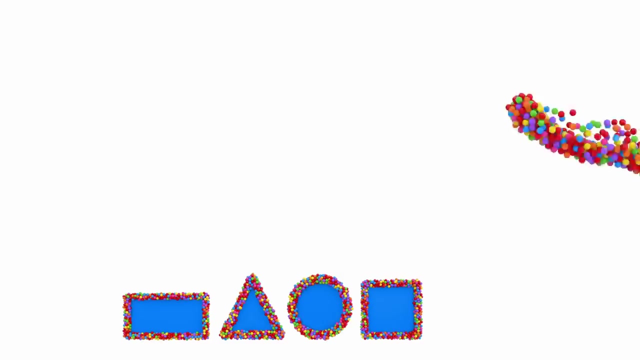 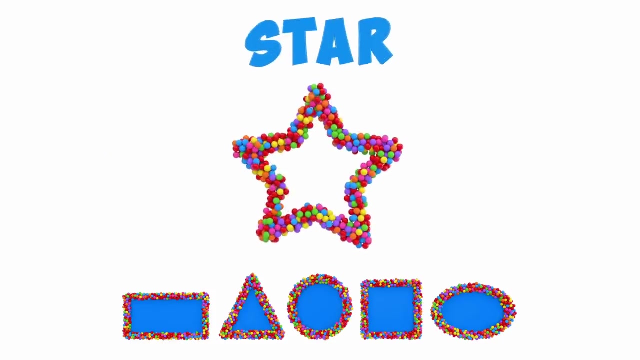 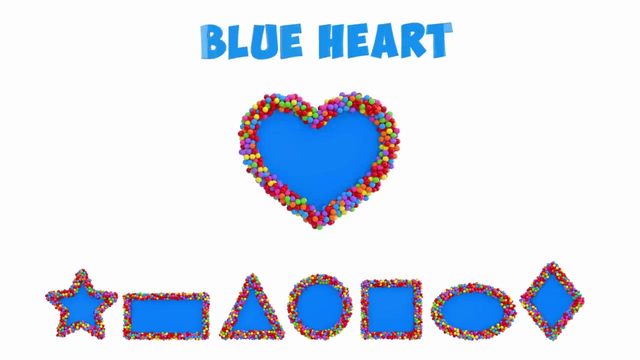 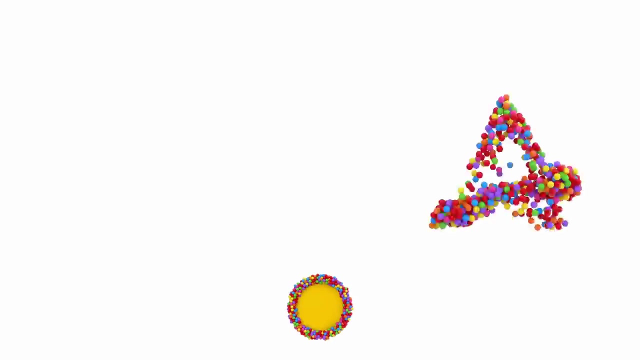 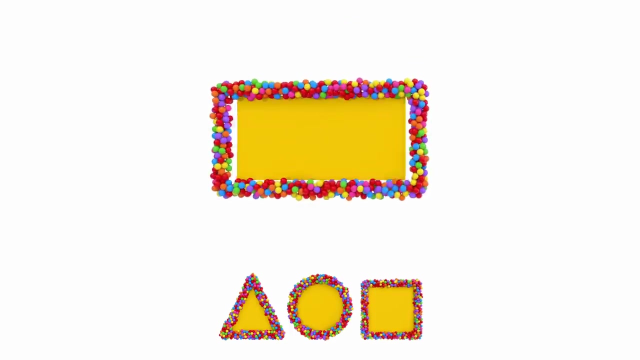 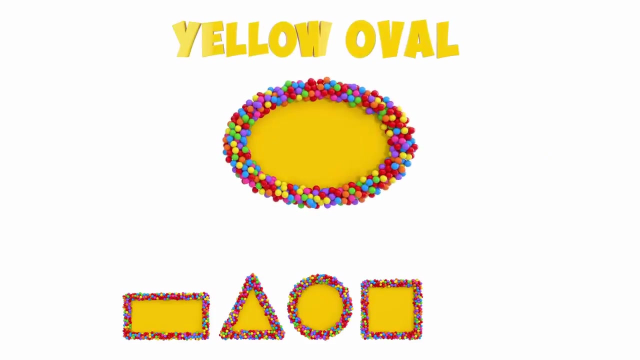 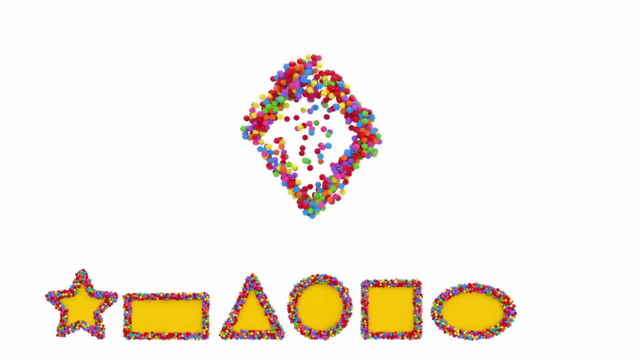 Red heart Circle. Blue circle, Triangle. Blue triangle Square. Blue square Rectangle. Blue rectangle, Oval. Blue oval Star. Blue star Rhombus. Blue rhombus, Heart. Blue heart Circle. Yellow circle, Triangle. Yellow triangle Square. Yellow square Rectangle. Yellow rectangle, Oval. Yellow oval Star. Yellow star Rhombus. 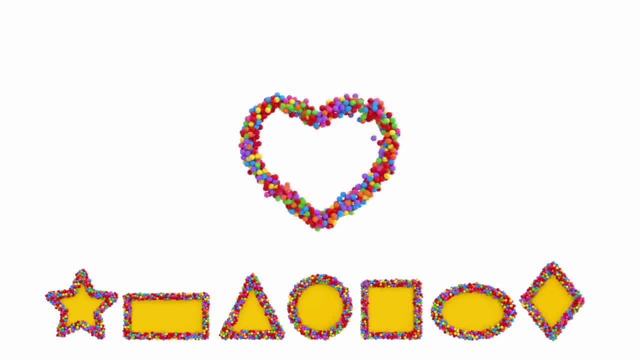 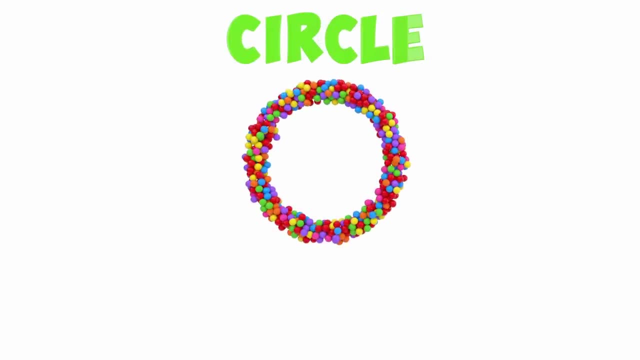 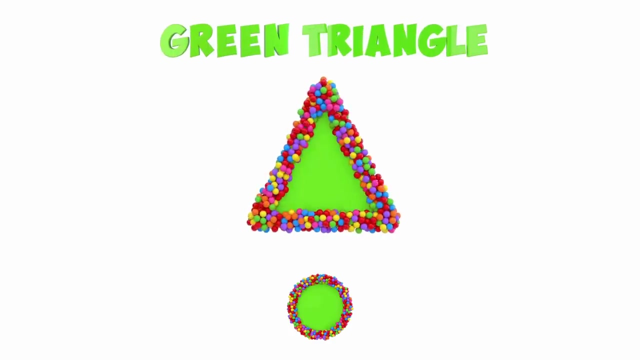 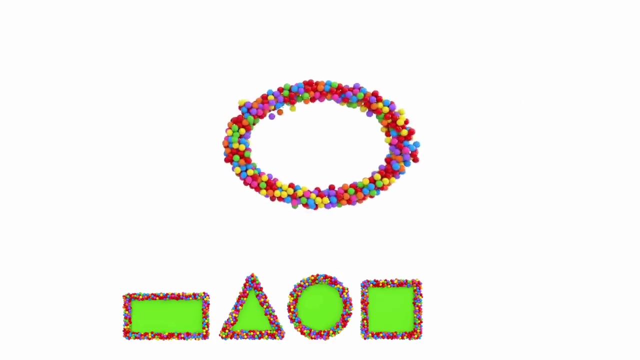 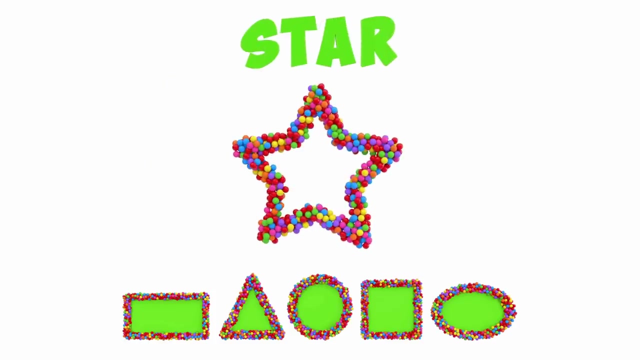 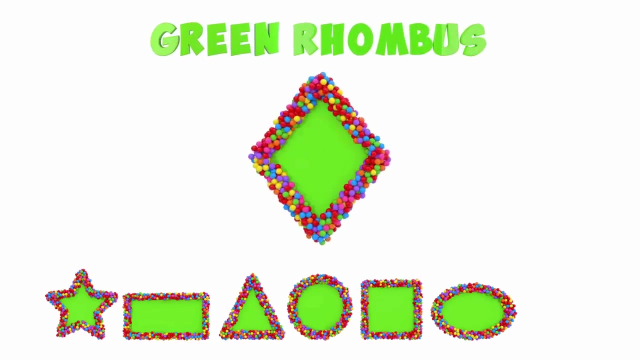 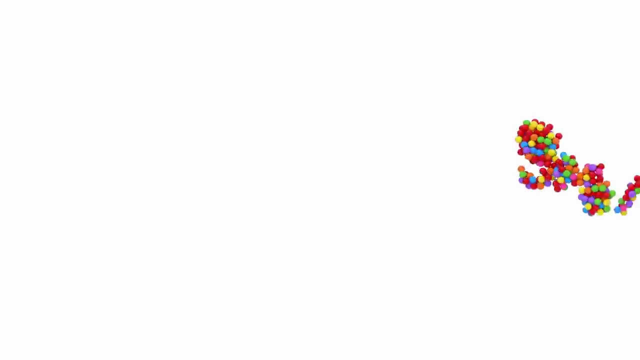 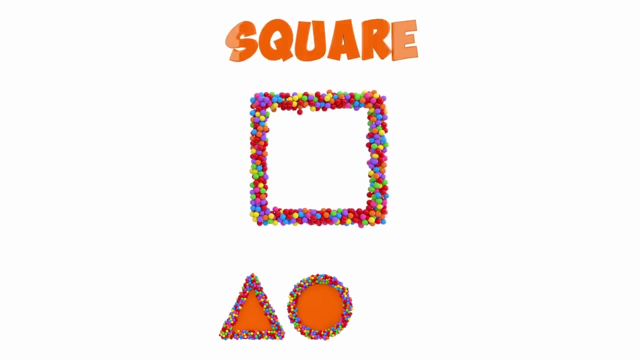 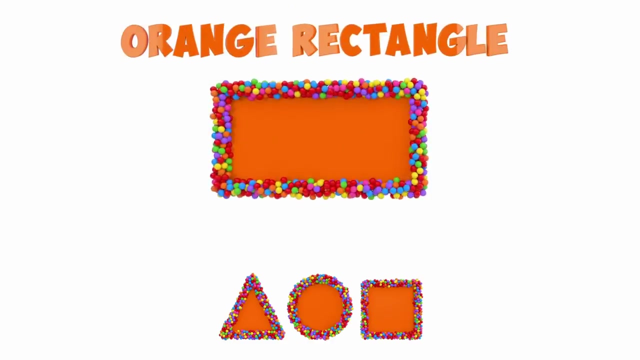 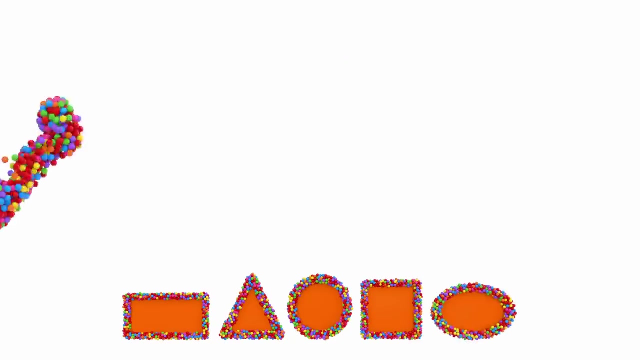 Yellow rhombus Heart, Yellow heart Circle. Green circle. Triangle. Green triangle Square. Green square. Rectangle Green rectangle. Oval. Green oval Star. Green star. Rhombus Green- rhombus Heart. Green heart Circle. Orange circle. Triangle. Orange triangle Square. Orange square. Rectangle. Orange rectangle Oval. Orange oval Star. 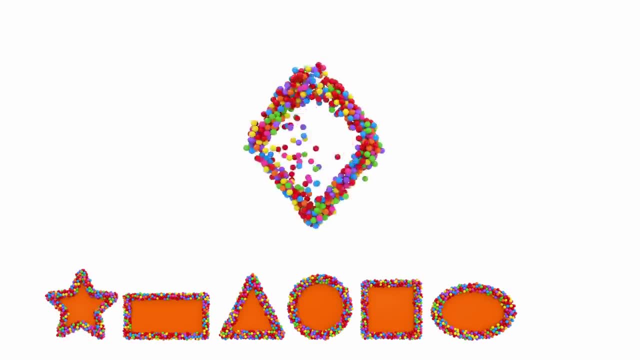 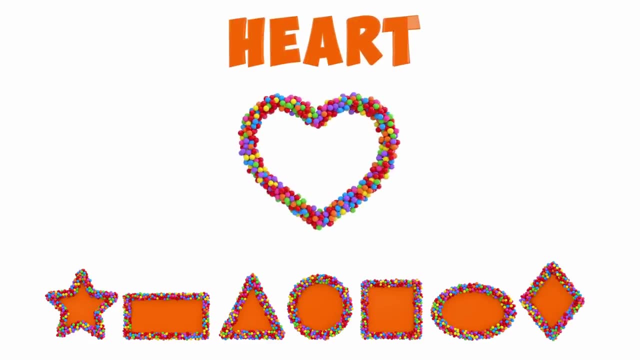 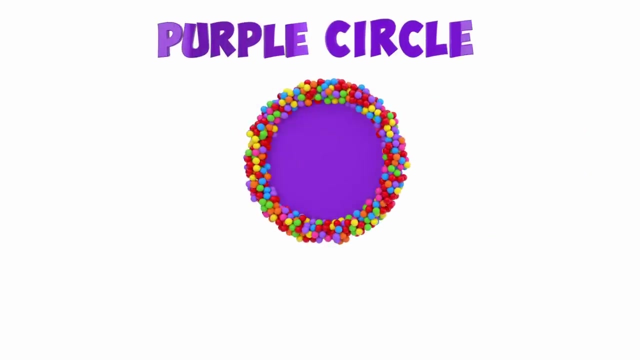 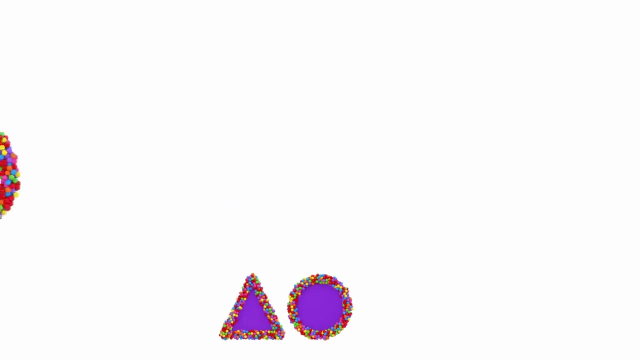 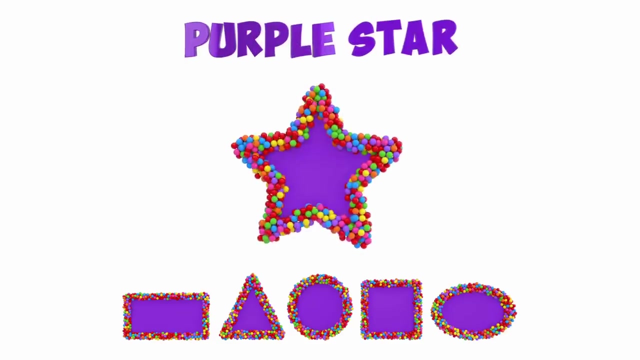 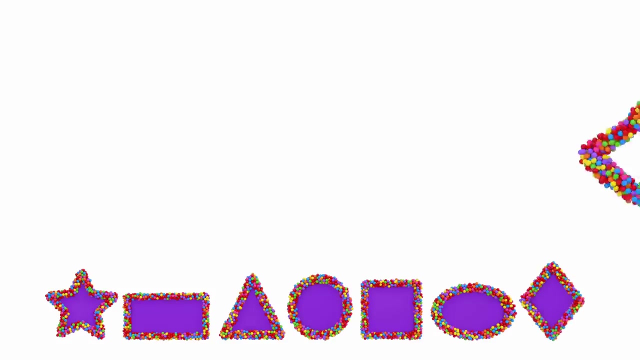 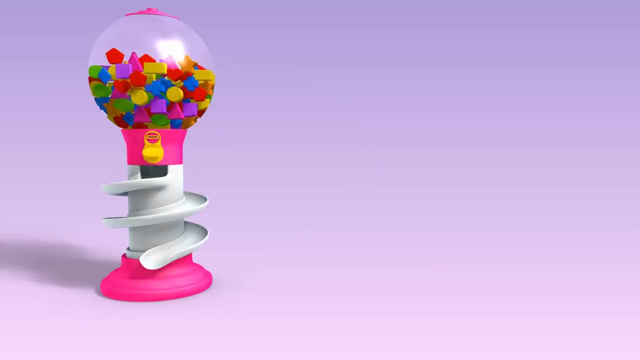 Orange star, Rhombus. Orange rhombus Heart. Orange heart Circle. Purple circle, Triangle. Purple, triangle, Square. Purple square, Rectangle. Purple rectangle, Oval. Purple oval Star. Purple star, Rhombus. Purple rhombus Heart. Purple heart Circle, Heart Circle, Circle, Square, Square, Triangle, Triangle, Triangle, Rectangle. 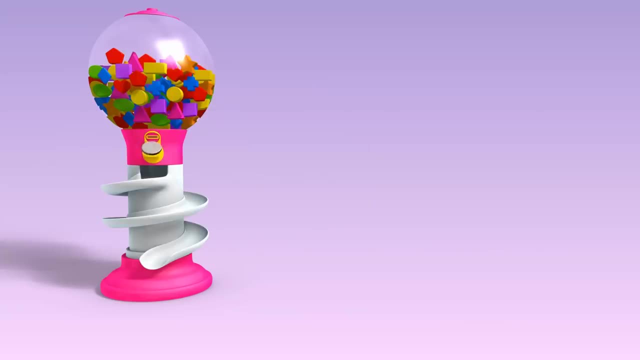 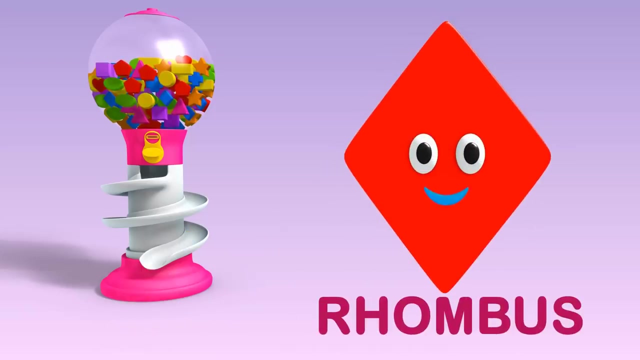 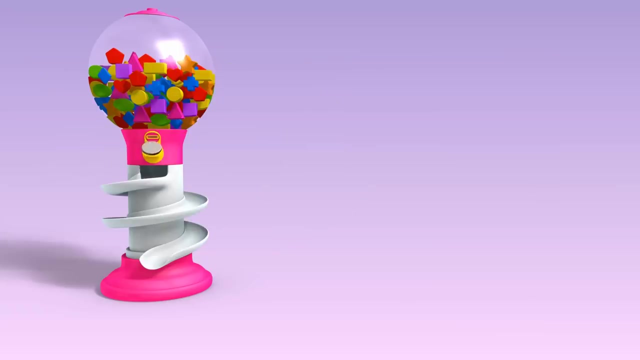 Rectangle, Oval, Oval Parallelogram, Parallelogram, Rhombus, Rhombus, Heart, Heart, Star, Star, Crescent, Crescent, Arrow, Arrow, Cross, Cross, Crescent, Divide Cross, Pentagon.